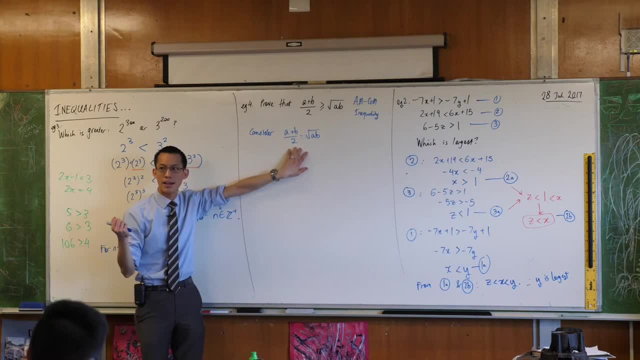 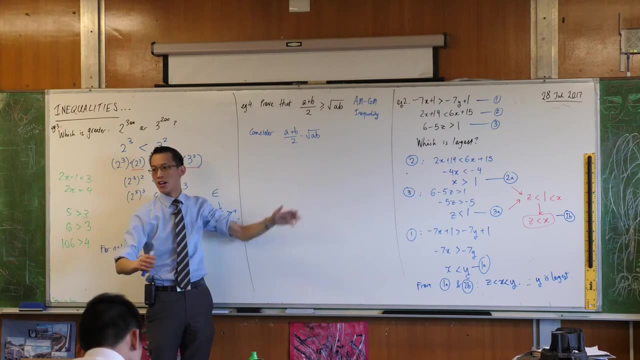 then this is what I would get on the left-hand side. What will be left on the right-hand side? 0.. So I want this thing to be greater than or equal to 0, so I don't want it to be negative. is what I'm saying, okay? 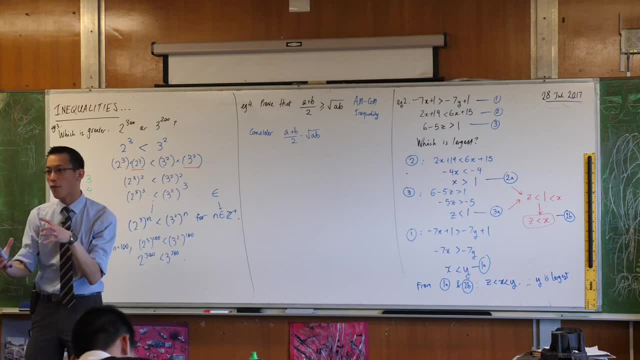 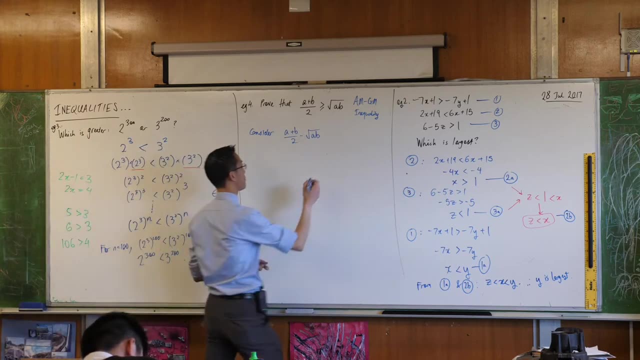 So if I can muck around with this and twist it into a form to demonstrate, this thing has to be greater than or equal to 0.. zero. then I'm home, okay, So here's what I'm going to do. I admit that this doesn't. 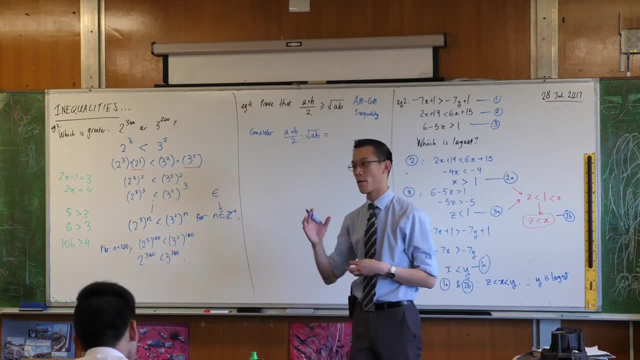 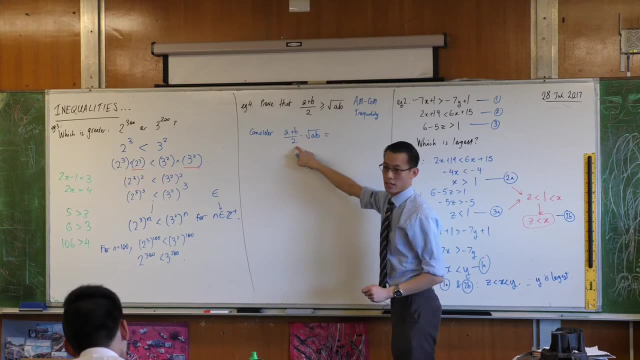 look intuitive at first, but I'm going to borrow some of the knowledge from our idea of factorization from before to try and get this thing together. So first step: You have two things. one's a fraction. What do you normally do when you've got two things and 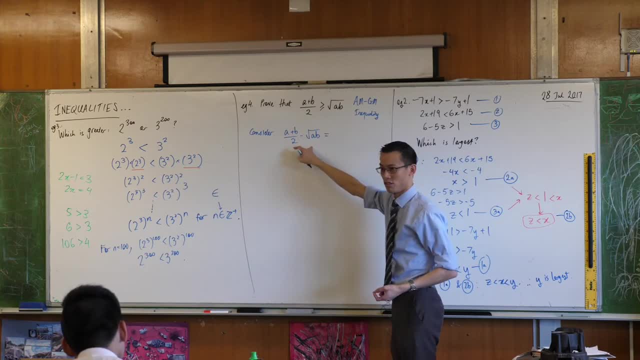 one's a fraction. You just combine them right And then you've just got one fraction. One fraction is better than two fractions, So that's going to be a plus b. take away what when you get on that common denominator, 2 square root ab, like that. okay, I'm going. 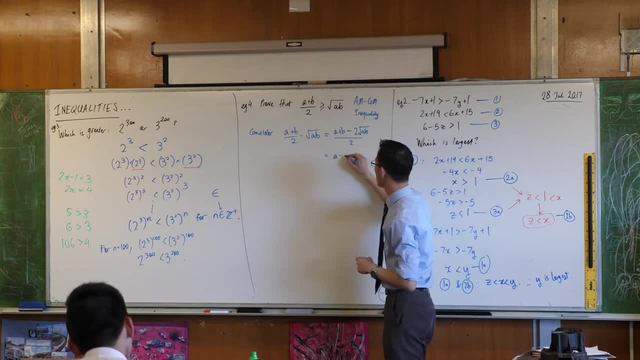 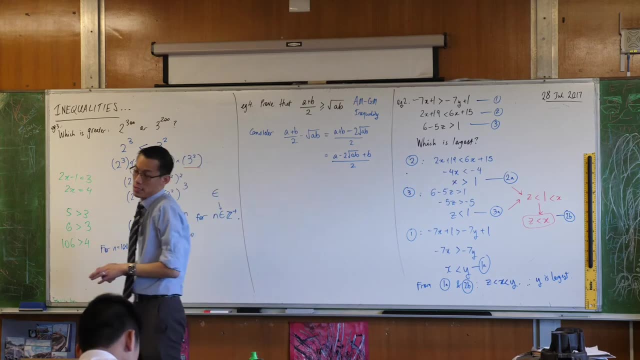 to shuffle it just a little bit to see if this helps you to spot that this is something that you've seen before. I'm going to write it like this: which seems like it's no different, right? Because it isn't different: it's the same thing, But that numerator there, that. numerator is something you've seen before, So I'm going to write it like this: which seems like it's the same thing. But that numerator there, that numerator is something you've seen before, So I'm going to write it like this: which seems like it's the same. 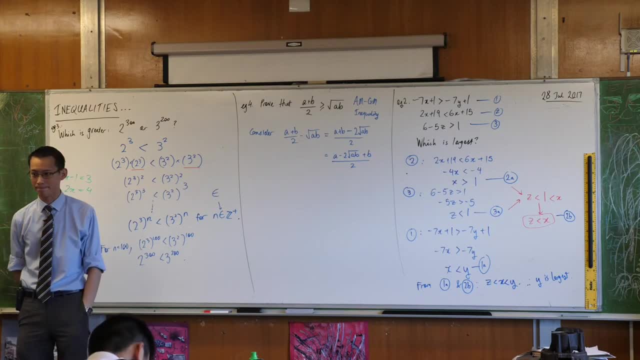 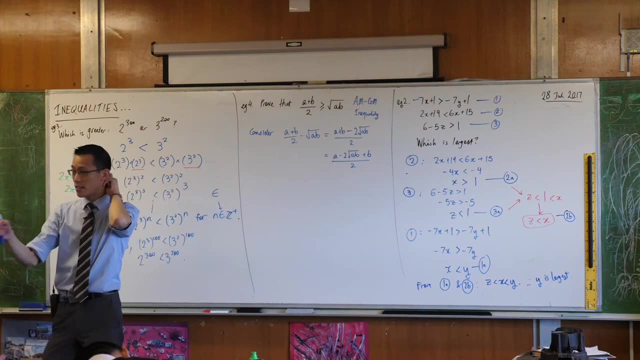 thing. But that numerator there. that numerator is something you've seen before. It's just dressed up a little bit differently. Something minus two other things plus something else. Something minus This is a square, isn't it? Now, maybe it's not immediately like. 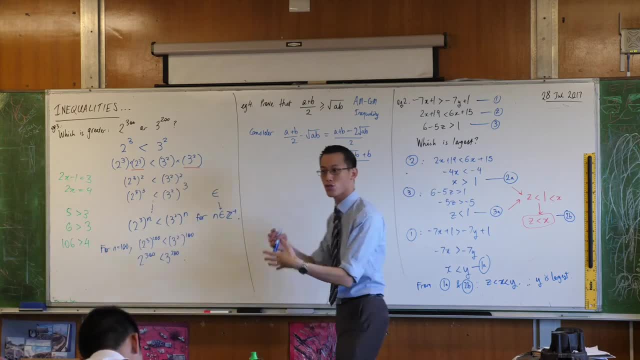 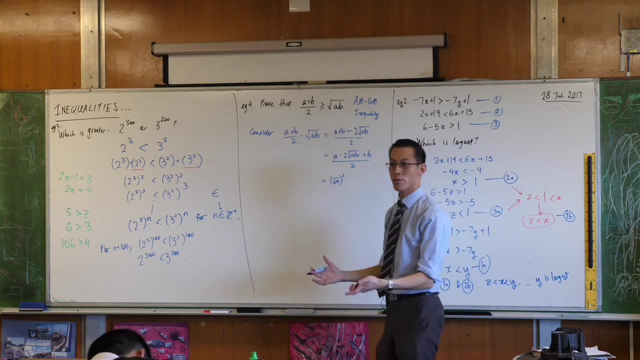 what do you mean? What square is there? Let me rewrite it again to try and clarify that it's a square. a is the square of the square root of a right Like this would give me this By the same logic. b is the square of the square root of a right Like this would: 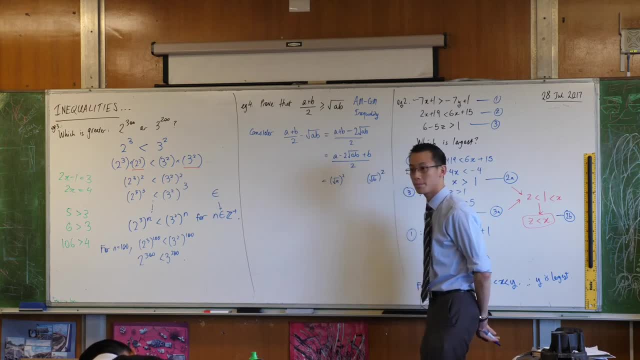 is the square root of b squared. yes, So this is actually square root of a, square root of b. The reason I thought of that is because I've got the square root of a and the square root of b in here, right? 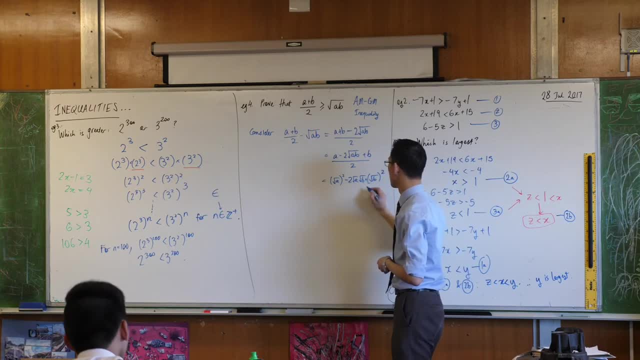 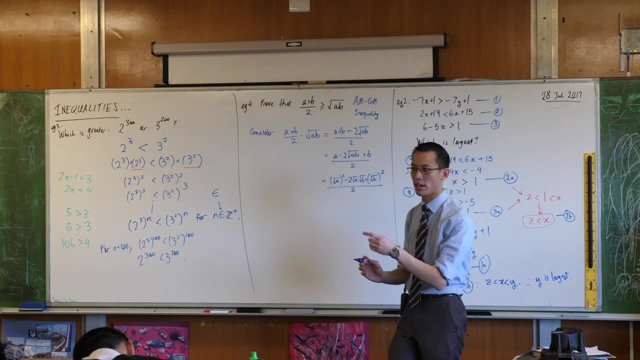 So this, in fact, is two lots of square root of a, square root of b. That's all divided by two. Now maybe it's a little clearer that this is a perfect square. What's going to be in the brackets? It's root a minus. 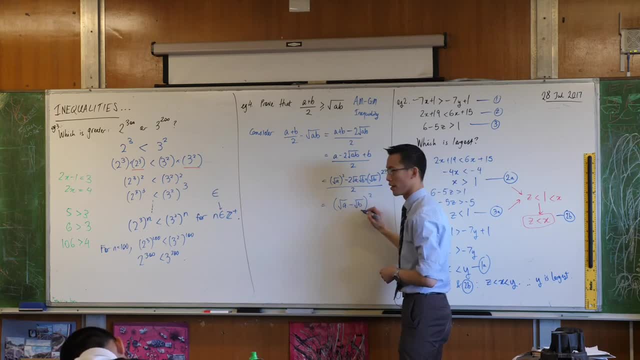 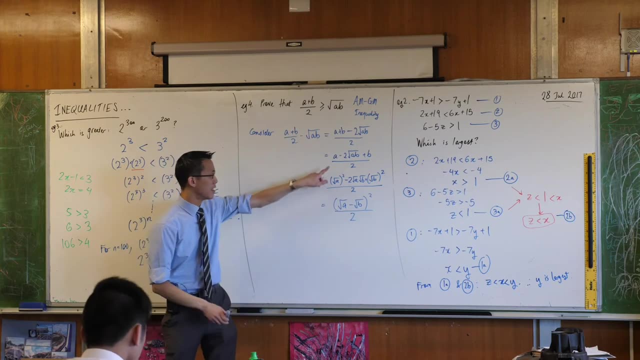 It's a minus because of this guy right The square root of b. Yes, are you happy with that? Now, I pushed you in that direction to try and say to you: hey, hey, hey, this is something that you know. 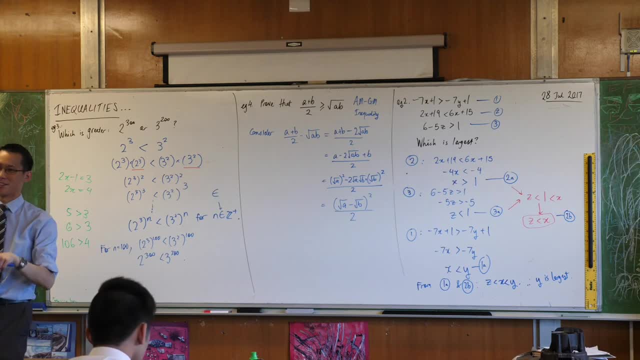 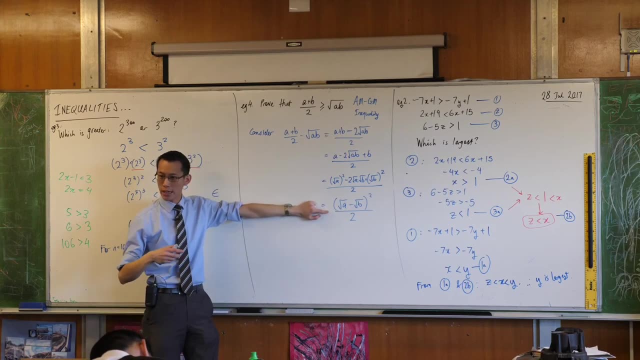 but obviously you're going to encounter questions like this and you don't have me pushing and prodding you and like a little voice on your shoulder. So one of the skills you're practicing here is: things often are things that you know about, but we intentionally 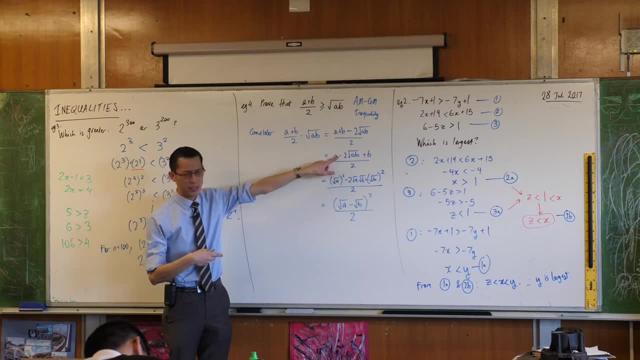 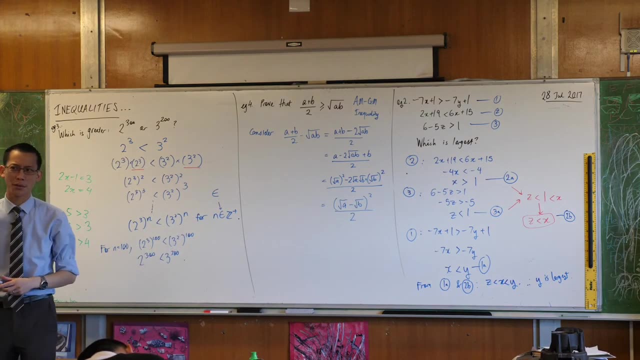 We intentionally try and obscure those to see. do you really recognize, Do you really see that there's a pattern here that you've actually been using for years now? Okay, what was I trying to prove? again, Go back to the beginning. What was I trying to prove? 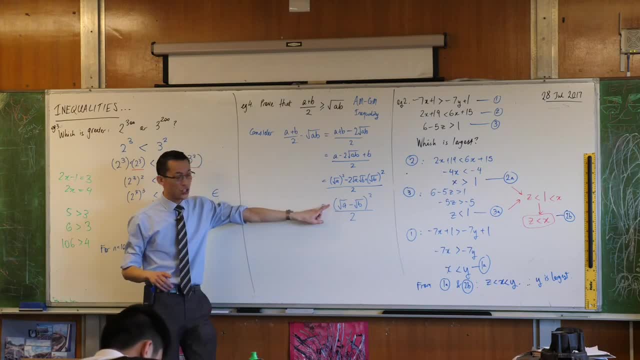 Yeah, bigger than or equal to zero, right? Do you see, I've pretty much achieved that right, Because, look, you've got a number, take away a number and then you square it right. Well, in the numbers that we know about. 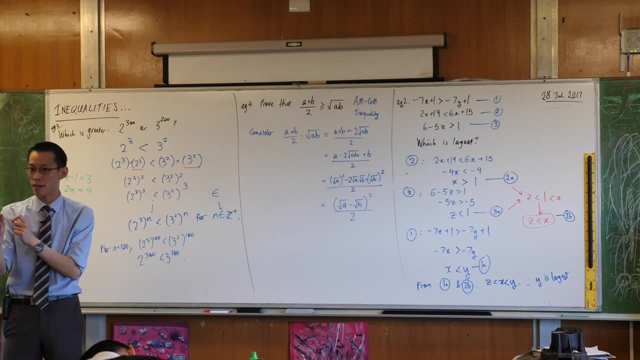 that thing has to be Like: the smallest that could possibly be is zero. That's what. That's what square numbers will do. There are numbers that you square, you get negatives, but we're not dealing with those at the moment. okay. 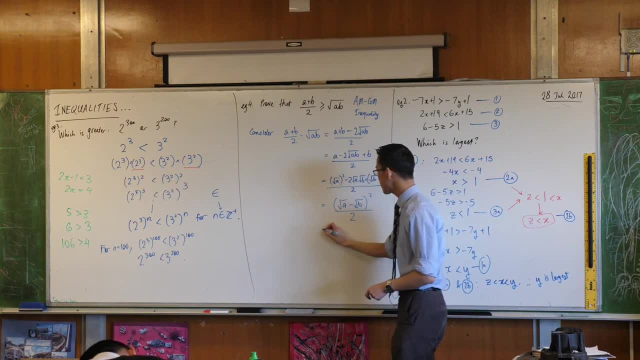 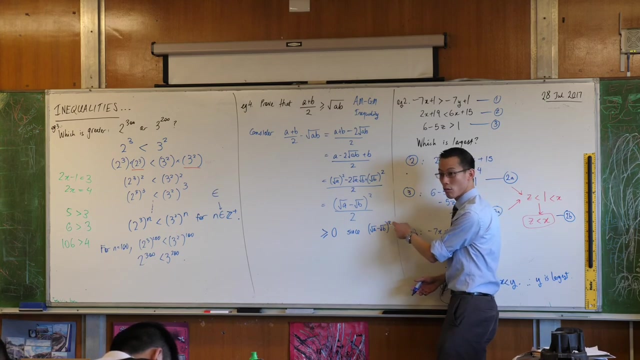 So therefore I can say: this thing here is greater than or equal to zero. since this guy here that has to be greater than or equal to zero. Does that make sense? It's a square right. So the smallest it could possibly be is zero. 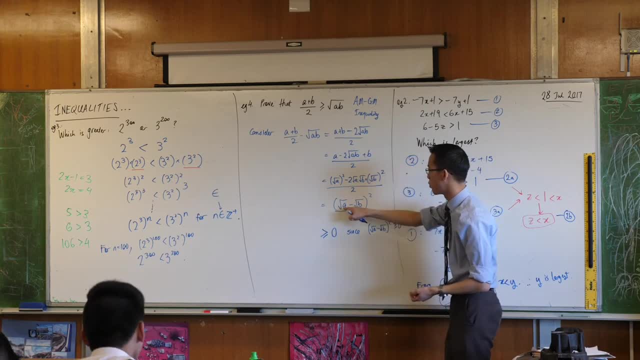 but it's very likely larger than that. okay, No matter what number you put in for A and B, so long as they're- Excuse me, The numbers we've been dealing with all along- root 5 minus root 2,. 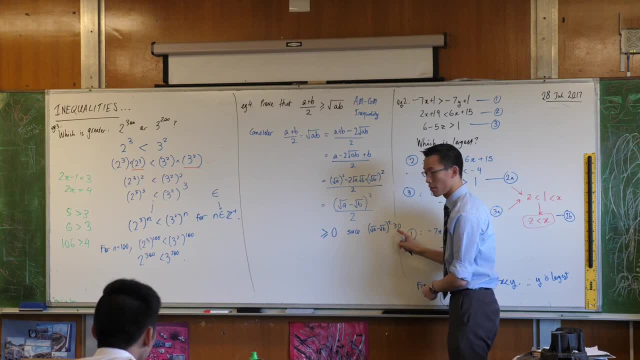 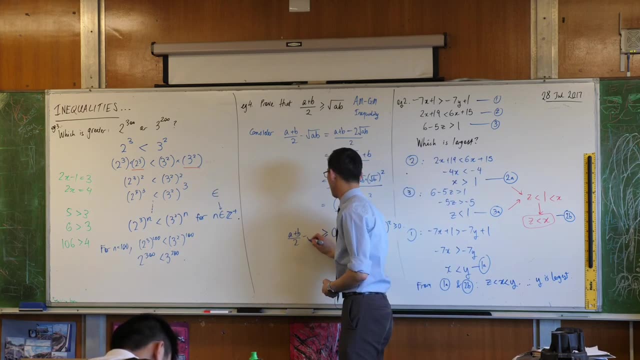 root 100 minus root pi. whatever you like you square it, you'll get something that obeys this law. Dividing it by 2 doesn't change that. So now I have this, because that's what was on the left-hand side all along. 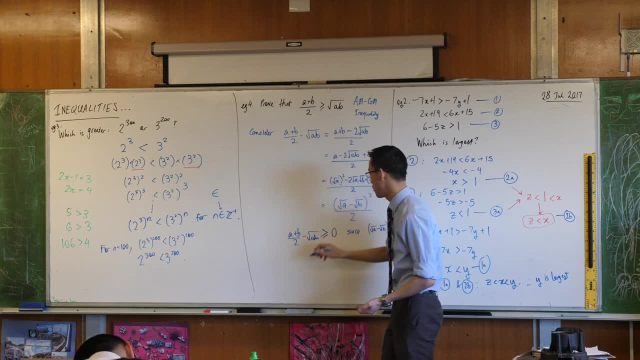 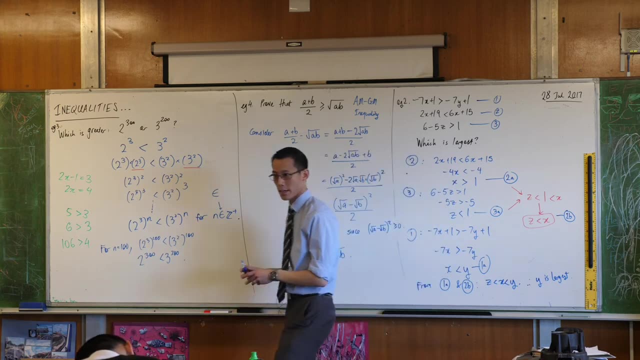 and so it's only one step to get to the actual result that I was supposed to prove. Therefore, this is bigger than this. Okay, So that's kind of handy.